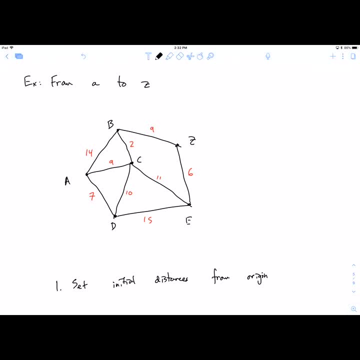 as quickly as possible. So the way Dijkstra's algorithm works. it's simple to write down, but we'll run through a couple examples to get a sense of how this works. So at the beginning of the problem you first set initial distances. So for each node in the graph, 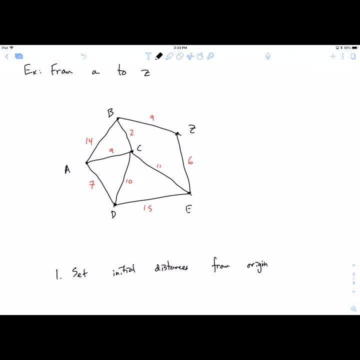 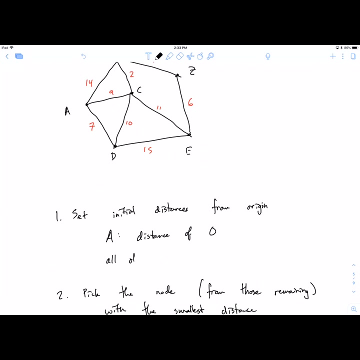 we're going to set an initial distance, And the way we do this is: a gets a distance of zero, meaning that's where we're starting. So from the origin, since a is the origin that gets the distance of zero from itself, and then everything else. we set the distance to infinity. In other 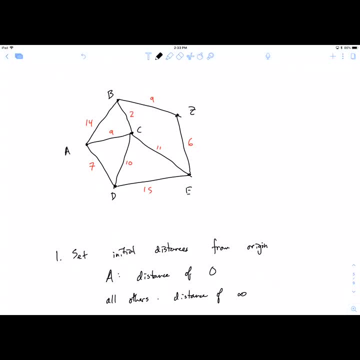 words. as things stand, to begin, we just set it as a huge number, and the goal is we're going to cut these distances down by finding shorter paths to each one of them. So we start with the distance of 0 at A, and then everywhere else we mark. 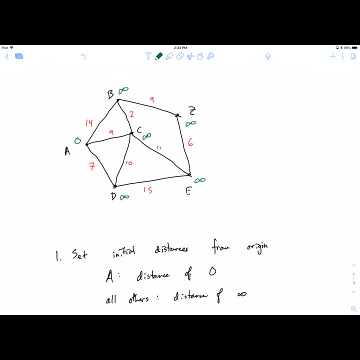 with infinity, just to begin with. So you'll see, as we go through this, why we do that. but again, the idea is basically: at each stage we're going to look to see if we can find a shorter path to each node and of course, we can find something. 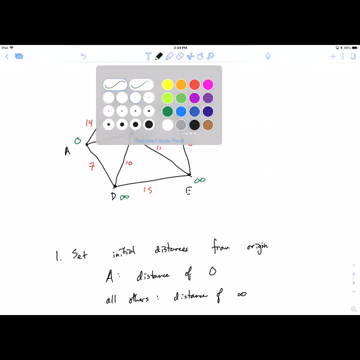 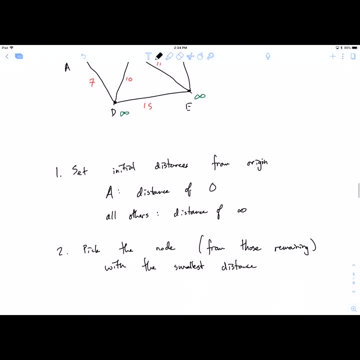 shorter than infinity to any one of them. So that's, that's how you start it out. and then the process of the algorithm: the, the part that gives the algorithm the name of an algorithm. the repeated step that you go through is you pick the node from all those remaining that has the 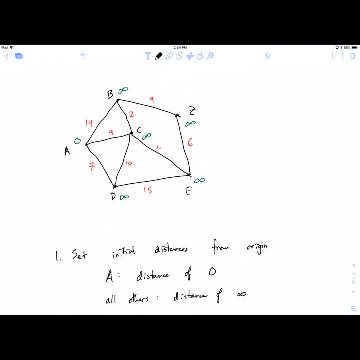 smallest distance currently. So on the first step, you would pick A, because that has the smallest distance of all of them. the others are infinity. So you pick the one with the smallest distance and then what you do is you update the distances to all their distances. 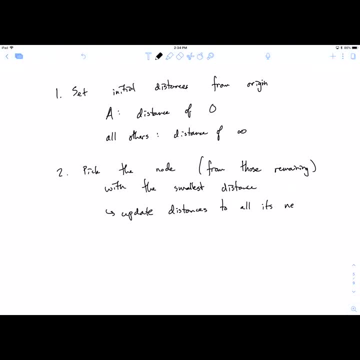 All their neighbors, all its neighbors, Meaning you look to see, can I find a shorter path from this point to its neighbor than what it currently has? You'll see that as we go through and practice how this works And then, once you've done that, you check off that node, meaning you've finished with it. You've. 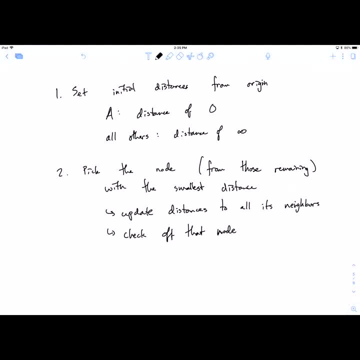 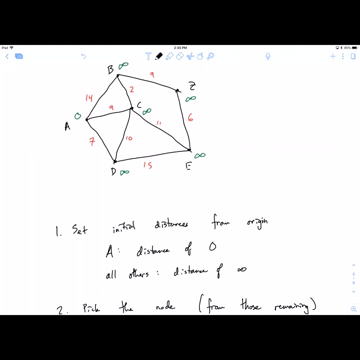 visited it, you've checked it. you don't need to come back and look at it again And then you repeat this until all the nodes have been visited. So the idea is we just, instead of accounting for all possible paths from A to Z, we just have to account for all the nodes in the graph, which is a much 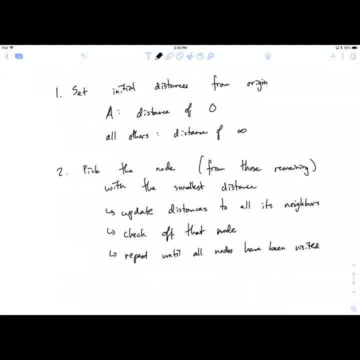 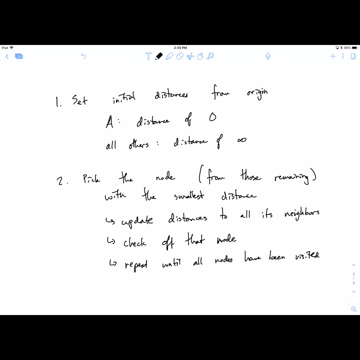 smaller number of things to account for. So that's kind of the the beauty of this algorithm that it gives us that shortcut. So let's actually see this in practice, because just seeing the steps written out like this is not nearly as instructive as seeing an. 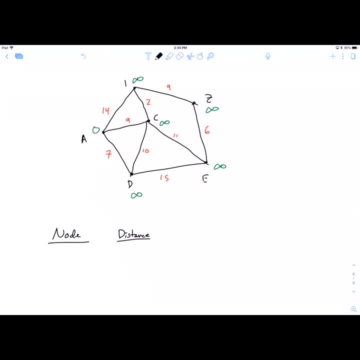 example. So we'll take this example- and I've drawn it again for you- with the initial distances set from A to each one of them. So these distances that are listed are the distance from A, the shortest distance you've found so far. So 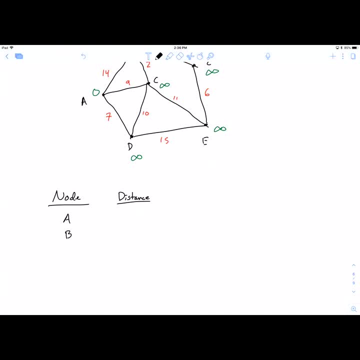 what I'm going to do here is list out the nodes. So we have A, B, C, D, E and Z, And And then the current distance of each of them. they're starting out at infinity- everything other than A. 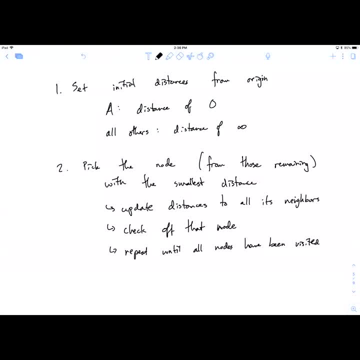 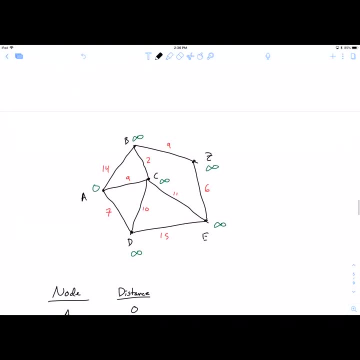 All right. so the algorithm says: pick the node with the smallest distance. so that would be A currently, update the distance to all its neighbors and then check it off. So what we're going to do is we're going to say: the neighbors of A are B, C and D, right? 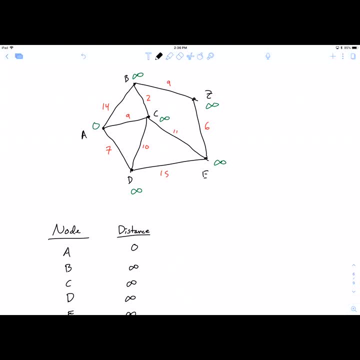 These are the ones that border A that are connected directly to it. So we're going to update the shortest distance we can find from A to each of those points, which would be the direct path to each one. So B, we can get there from A with a distance of 14, so we'll cross this off and say we 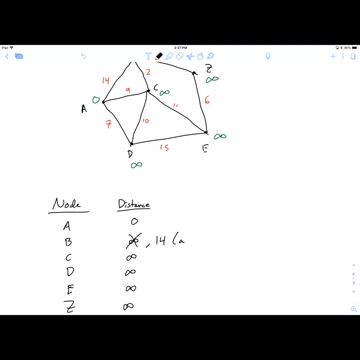 have 14 by going A to B, Then I guess I'll do it this way. Then B, C gets the same treatment. So rather than infinity we can find a shorter path which will get us there in 9.. And then D has a distance of 7.. 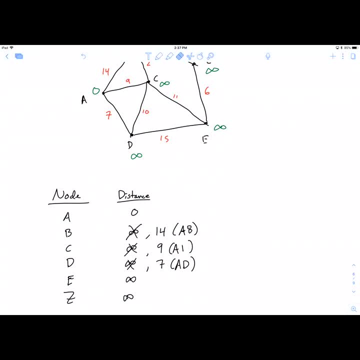 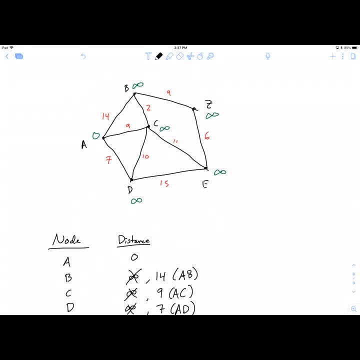 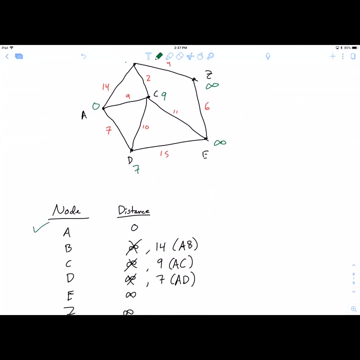 Sorry, this should be AC All right, so we can get directly to each one of them. So I'm going to erase these current weights, current distances, and replace them with 14, and 7.. So now we can check off A as being done, and now we're going to select of all the nodes. 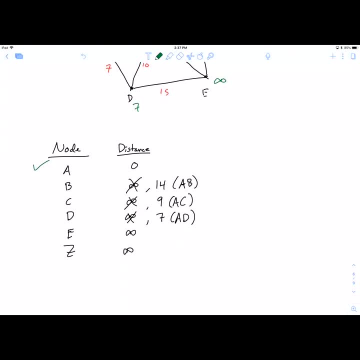 left that we haven't visited yet which one has the smallest distance. That would be D, And so we're going to repeat the process Now from D. we're not going to visit A again, because we're done with that one. 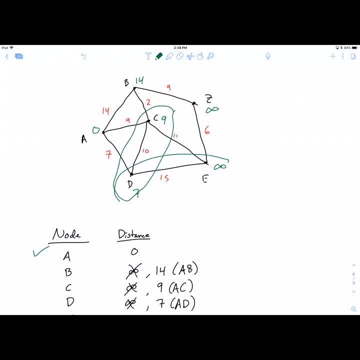 So we're just going to look at updating C and updating E and see if we can find a shorter distance. So we're going to go ahead and add this cost of traveling to C, and if that were shorter than going directly there, I would update it. 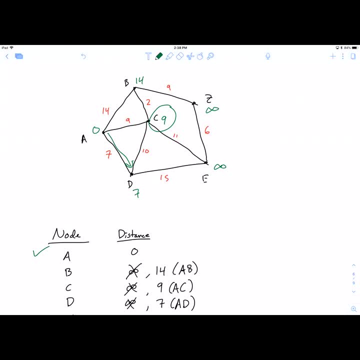 So in other words, if, Um, I got here with 7, and then say this only cost me 1,, then I would say: look, I can get to C faster if I do this than if I go directly there from A. 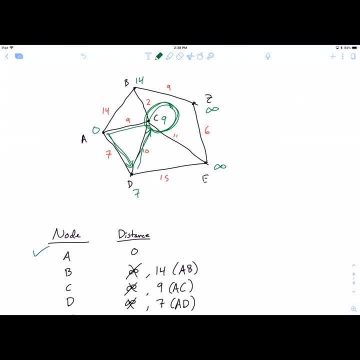 And so I would update the distance at C and say I can get there faster from passing through D. Now, that's not the case currently, because if I add the current D distance plus the additional 10,, I get 17,, which is not less than this. 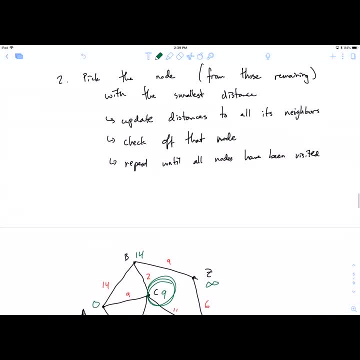 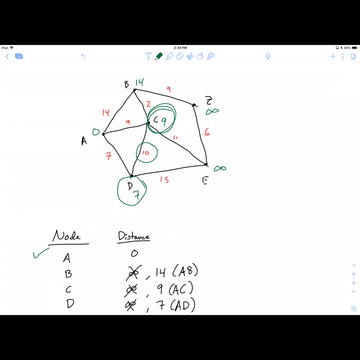 So I don't update that. So that second step, where we say we update the distances, what we're looking for is to see if we can find, See if the distance through the node we're interested in right now is shorter than the current distance to its neighbor. 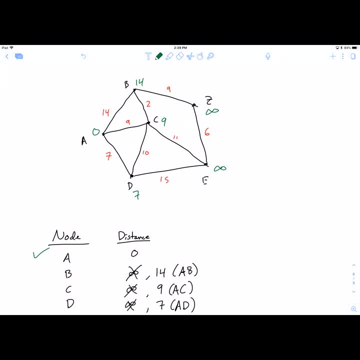 So that didn't make sense. We'll go through more steps so you can see it again. So C: we don't do anything with, we leave it alone. But E: we notice that from D we have A distance of 7 so far, and then an additional distance of 15, for a total of 22, which is 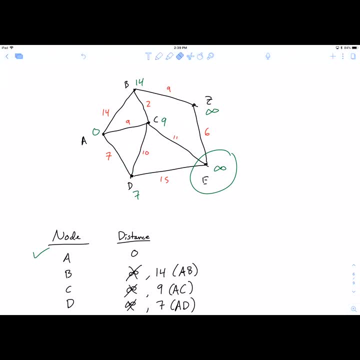 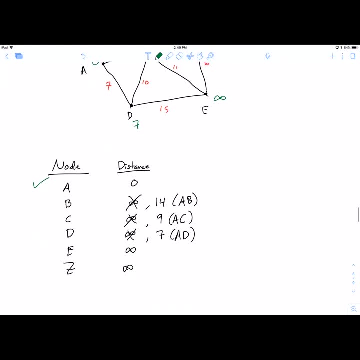 definitely less than infinity. And again, this is why we set the initial distances to infinity, so that they'll get initialized the first time they get checked. So E, we can get there in 22 by going A to D to E, So having checked all the neighbors of D, 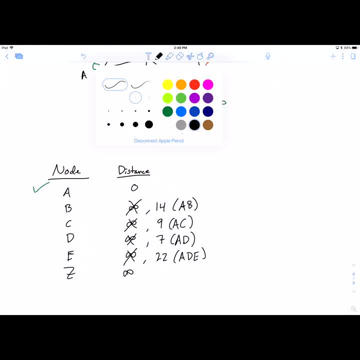 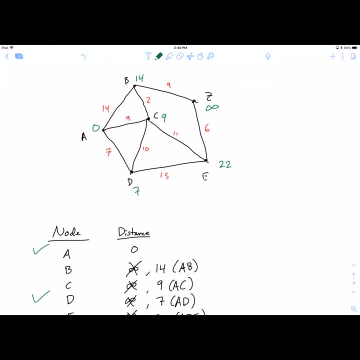 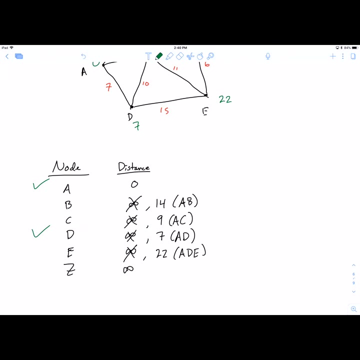 We check it off and we replace the distance at E with 22.. All right, so now we look through our list again and see which ones of the unvisited ones has the lowest current distance, and that would be 9 with C, but not with 9.. 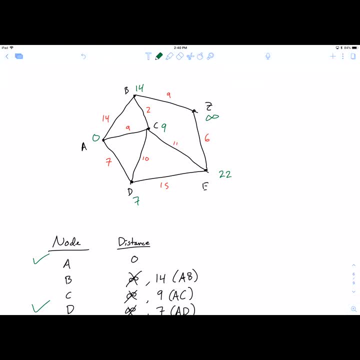 So we're going to go to C and we're going to check its neighbors. Now, we've already checked off A and D, so we're going to leave those alone. So we're going to go to C and we're going to check its neighbors. 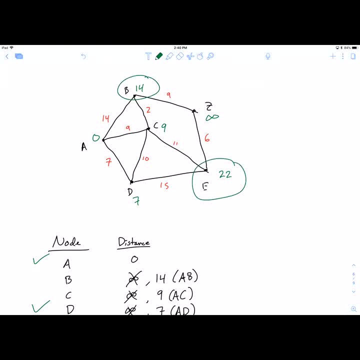 Now we've already checked off A and D, so we're going to leave those alone, But we'll check B and E and we'll see if we can get there to either one of those shorter than what the current best path to those is. 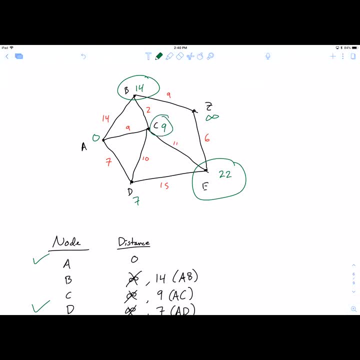 So from C if we go up to B, notice that we have 9. to get to C, An additional 2 costs us 11, which is better than the current 14 at B. So we're going to cross out the current. 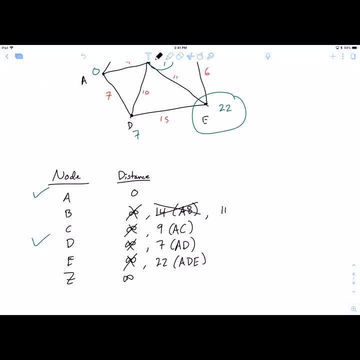 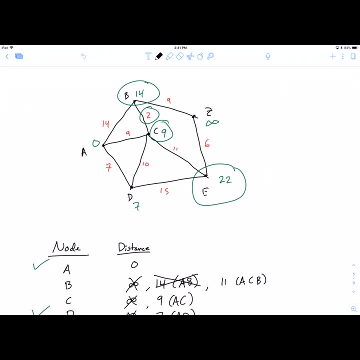 B And we have a total of 11 by going A to C to B. So it's faster to get to B by going through C than it is to get there directly. So going there directly costs 14, taking this side route costs 11.. 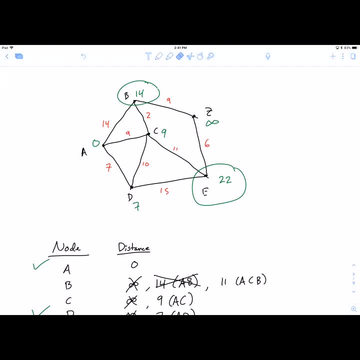 So we can update the distance there and say that's just going to be 11.. We can do the same thing to go to E. We've got 9 so far, So we're going to cross out the current 14.. We've got 9 so far. 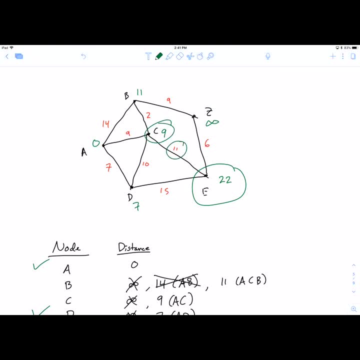 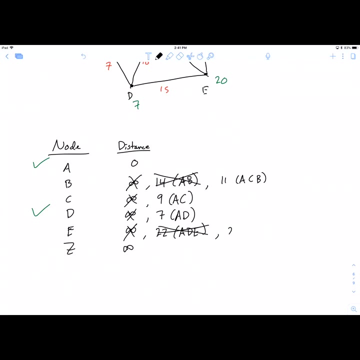 If we add 11, we'll get 20, which is better than the current 22.. So again, we're going to cross out the 22 and replace it with 20.. And that does the same thing here. So E we can do better than 22,. we can do 20 if we go A to C to E. 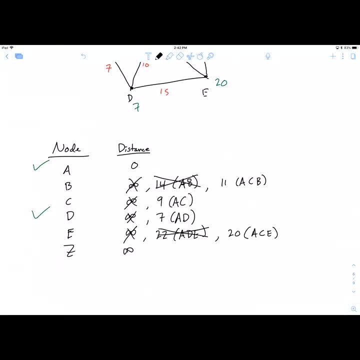 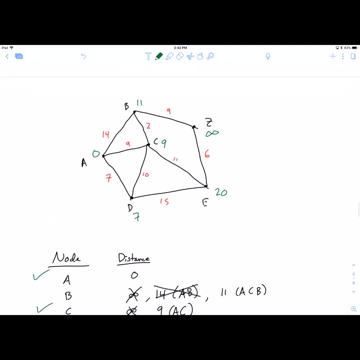 Having done that, we've checked all of C's neighbors And so we can mark off C. And now again we look through and say which of these unvisited ones has the lowest distance. There's only three left, And the lowest one we find is B, And so we go to B and check its neighbors. 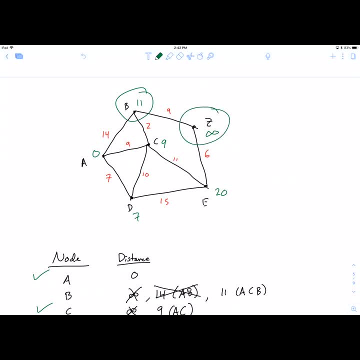 So the only neighbor of B that we haven't checked yet is Z, So we'll check that one. Since Z hasn't been visited yet, we'll certainly update that distance. The current cost of going to B is 11. And if we add 9,, we get a total of 20.. 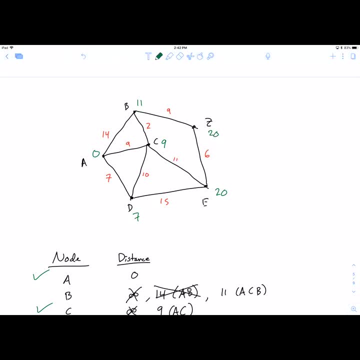 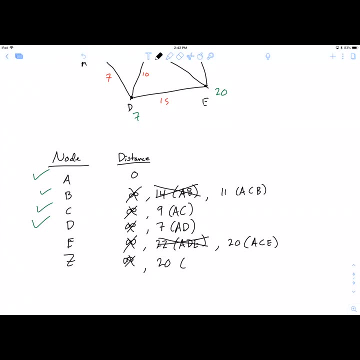 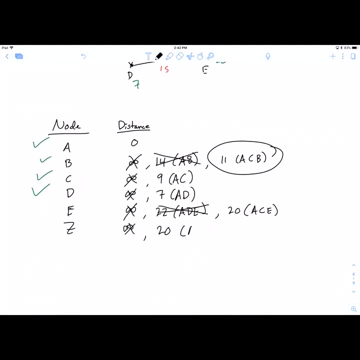 So we can get to Z with 20.. So we can check off B and we'll update the cost of going to Z with 20 by going Now. notice the shortest distance to get to B is going through C. So if we go A to C, to B to Z, that's currently the shortest route to Z. 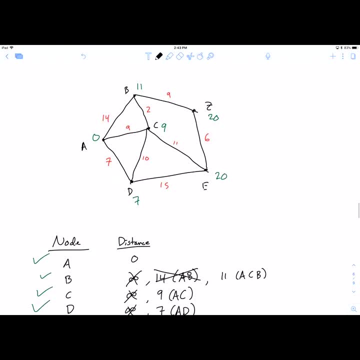 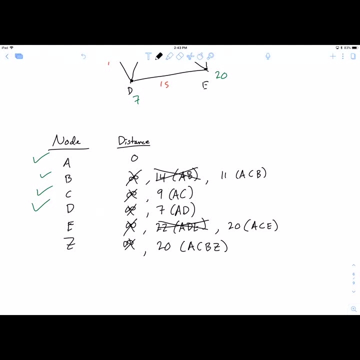 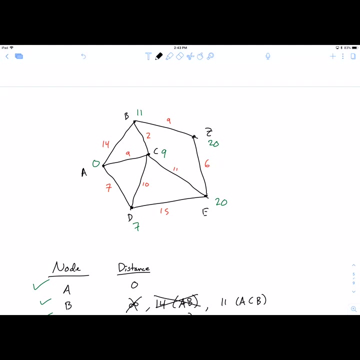 And then one last step. We'll check. We'll check going through E Now, if you notice. so that's our next lowest one that we haven't checked off yet. If you notice, the distance to E is already 20.. So going up to Z would add 6 to that, which is not better than the current optimal route. 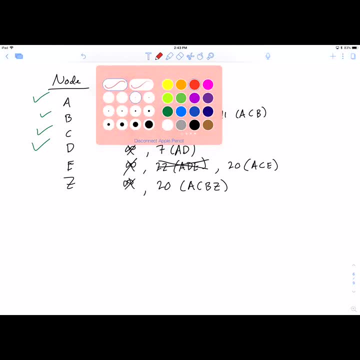 So the final answer is that our optimal route, the best path, would be to go A to C, to B to Z, and the cost is 20.. So that's really how Dodd-Dijkstra's algorithm works. in short, And again, it takes us longer to do it than it takes a computer to do it if you program it to do this. 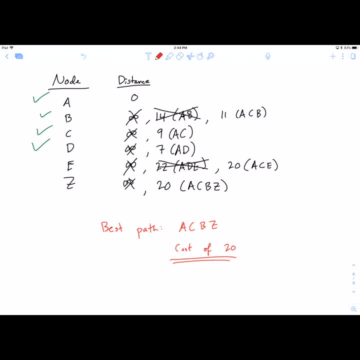 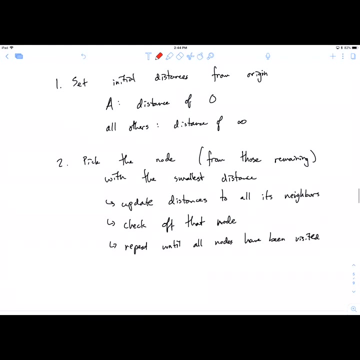 It's very efficient because we only had to really check a handful of nodes rather than accounting for all possible paths, which just very quickly gets out of hand. So there's our example of Our first example of seeing Dijkstra's algorithm at work. 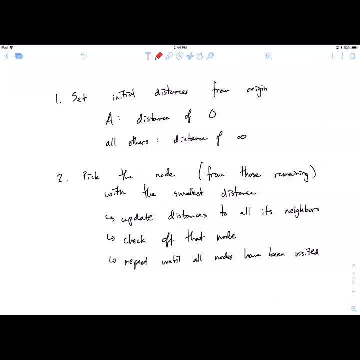 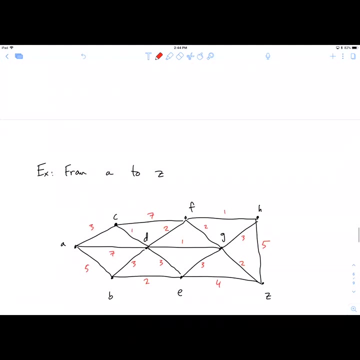 Here's the description of it: You start with the initial distances and then at each step you pick the smallest distance remaining and update the distance to all the neighbors before checking it off. So I want to do one more example, just to kind of drive this home again. 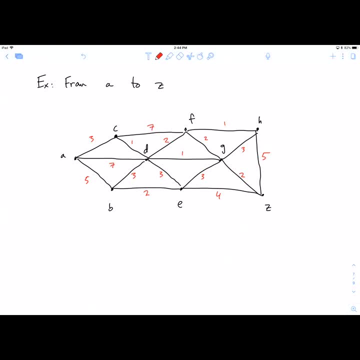 This one looks much more complicated And this, if you notice, there are lots of paths that would be possible through this little graph because it's so connected. There are so many connections going on here, But with this algorithm we can do it pretty quickly- about as quickly as we did the last one. 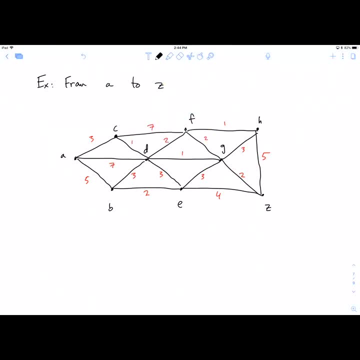 So I'm going to do something similar here, where I'm going to list out all of the nodes and we'll keep track of their current distance at each stage of the process. And so at the beginning we start out with 0 and infinity for all the others. 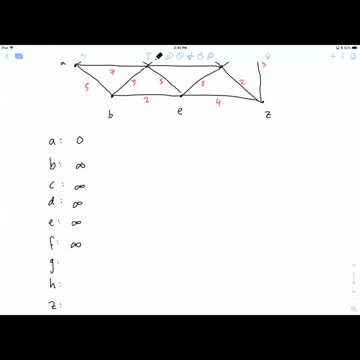 So again, we're starting at A and trying to get to Z. So all of these start out with infinity just as the initial value, and then we'll update as we go. So we start with A, the shortest current distance, and update its neighbors. 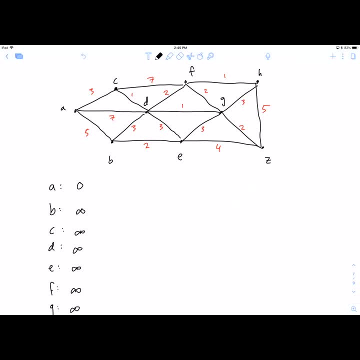 So the neighbors of A are C, D and B, And So we can update. B, for instance, has a distance of 5, if you go directly from A to B. C has a distance of 3, if you go directly from A to C. 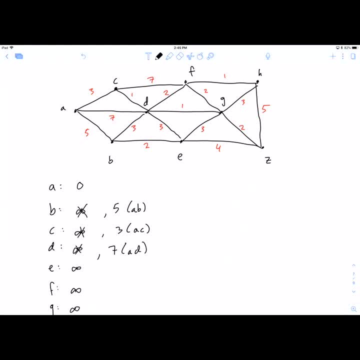 And D has a distance of 7, if you go directly from A to D. So then we check off A And of the smallest ones remaining, we notice C is the smallest one. So looking at C, what is it connected to? 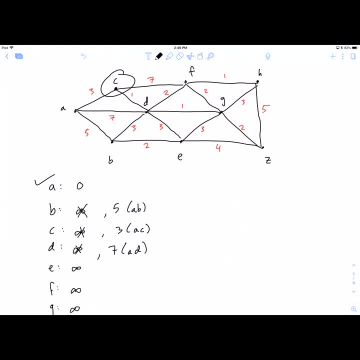 It's connected to A- We've already checked- And then D and F. So if we went from C from the current cost it has to D, that would add 1, which gives us a total of 4, which is better than the current cost that D has associated with it. 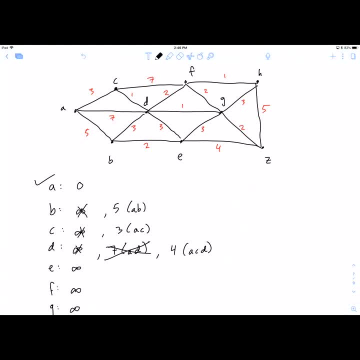 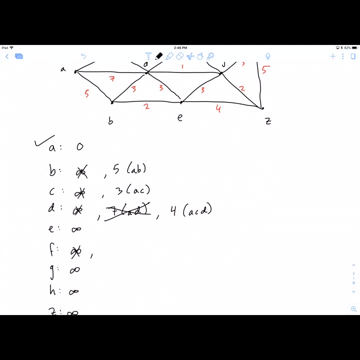 So if we go from A to C to D, we're better off than going straight from A to D And then from A to C to F would be a total of the 3 that C currently costs, Plus 7 to go from C to F, for a total of 10, which is better than infinity. 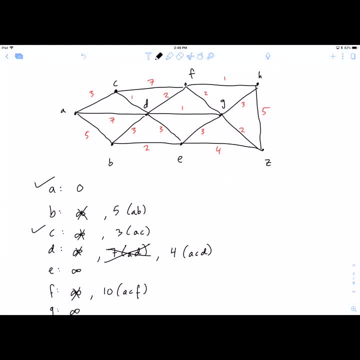 And then we can check off C, as being done. Then again, of those remaining, D is the smallest, So we can look into the neighbors of D D. we've already checked off A and C, so we're not going to go back there. 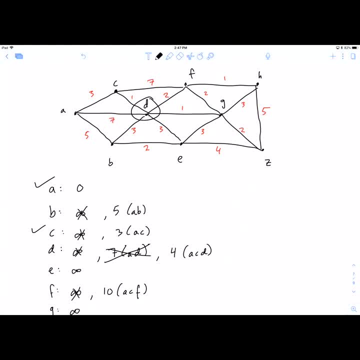 But we can go to B, F, G or E. So that's the first one, Next one: So again, I don't want to spend a lot of time going through the details here. If you go from D to B, that adds a total of 3, which gives you 7 total, which is not better. 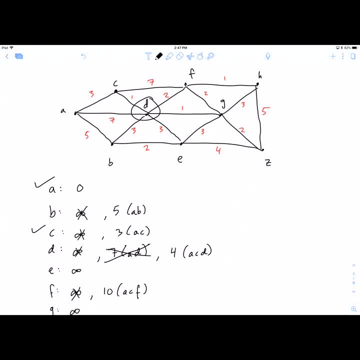 than the current distance to B, So we'll leave that alone. From D to F would give you a total of 6, which is better. So if we went from A to C to D to F, So we're taking this current path. 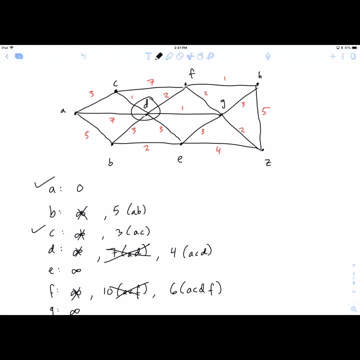 We're taking this current path to D and then just tagging on the distance to F And then to E, would be a total of 7, because we're adding 3 to get there. So that would be if we went from A to C to D to E, that would be a total of 7.. 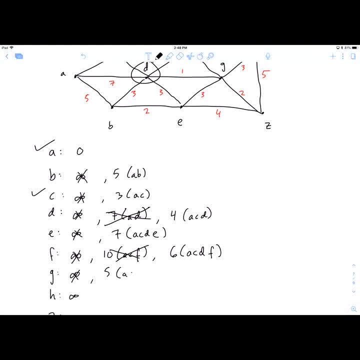 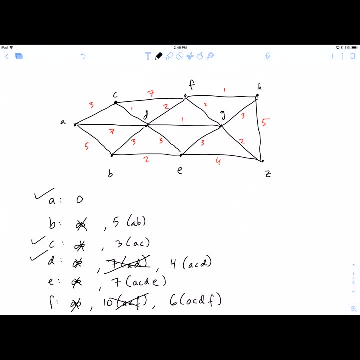 And then lastly to G would be a total of 5.. So we've done all of the neighbors of D, so we can check that off as well, And then just a couple more steps won't take too much longer, The shortest one that remains. 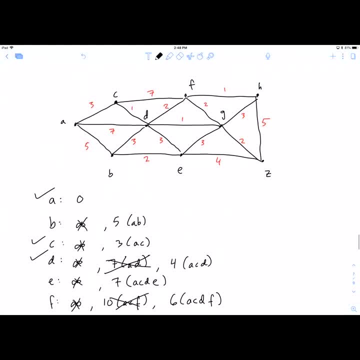 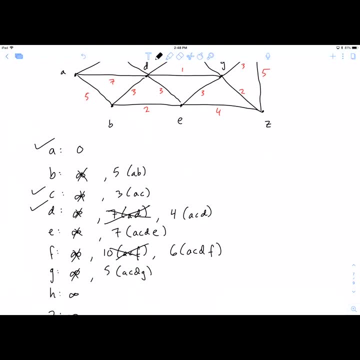 of the ones we haven't checked off yet is B. From B, the only neighbor we haven't checked off yet is E. That would be a total of seven, because we have the five currently to B and two more to get to E. That matches what we have currently, so we won't bother updating it. There's no benefit to updating. 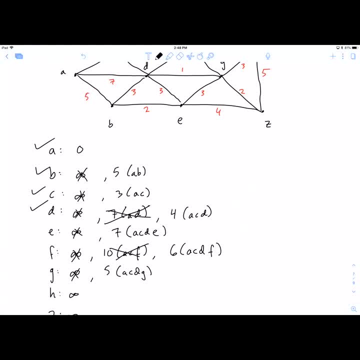 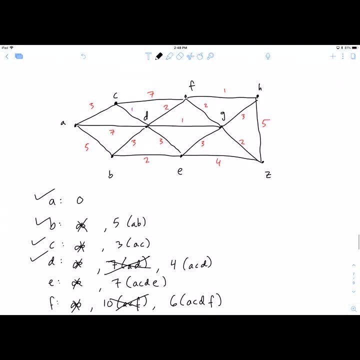 it, even if it keeps the same distance. So we'll leave that alone. check off B and we're done. The remaining smallest is G, so we'll check the neighbors of G. Notice that from G you can get to Z with two, you can get to E with three, you can get to F with two and H with three.